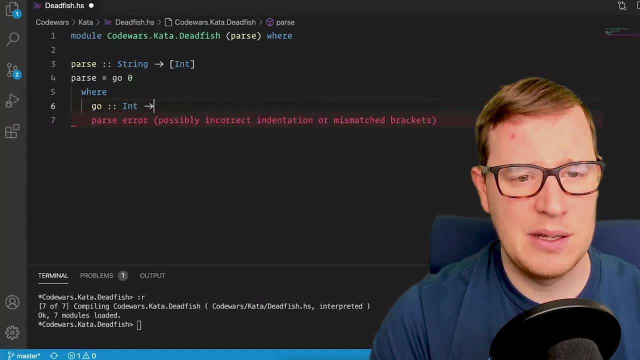 go where? go is a function that we're going to call go and it's going to start by zero. So we're going to define a function that we're going to call go and it's going to start by zero. So where is the function that is going to take an int, then is going to take a string? 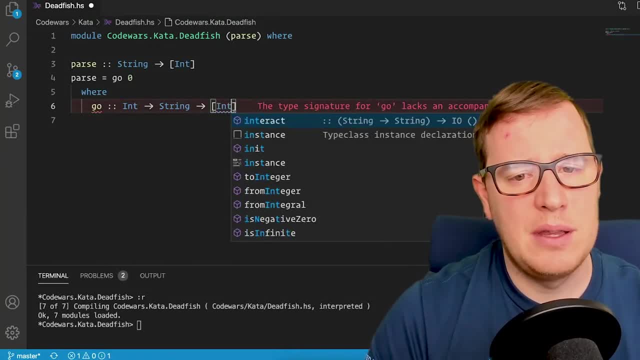 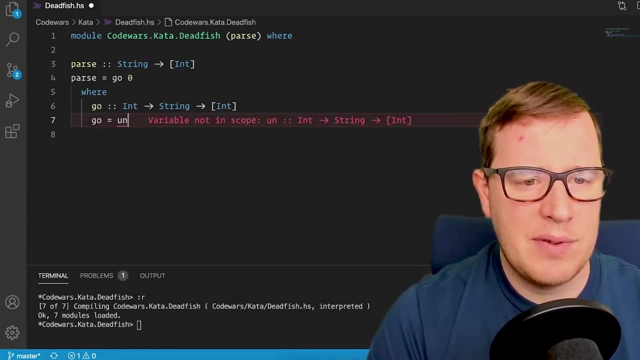 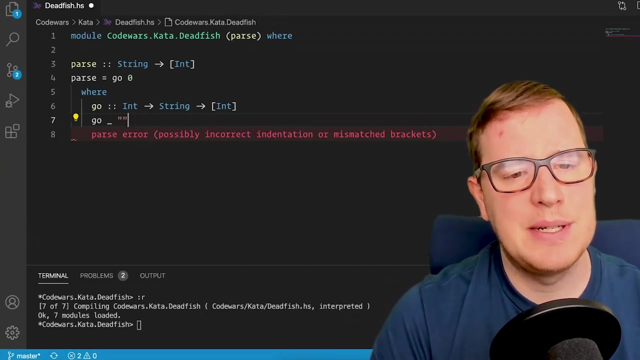 And finally, it's going to return the list of ints that we're looking for. So all good to go, And let's define what we want it to happen. If we are done parsing the string, we're basically. this is the stop case of our recursion. we're. 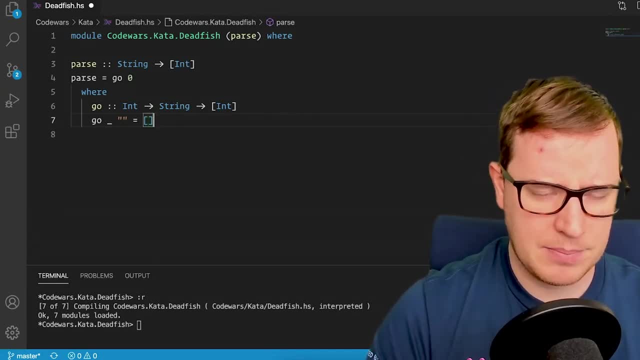 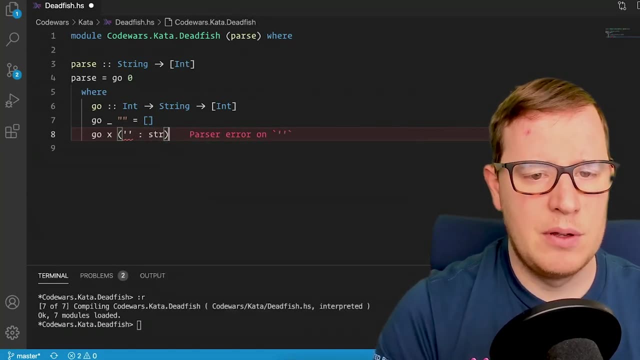 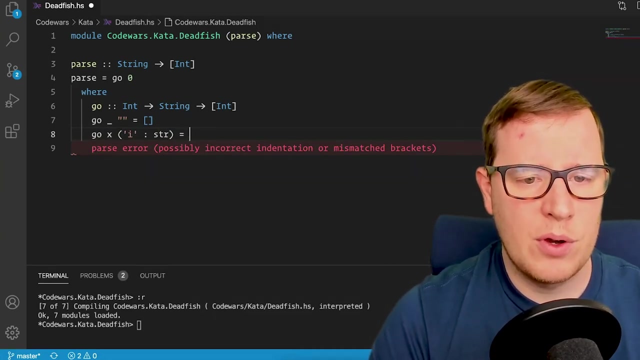 just going to return an empty list. If the command we want to interpret now it's i, we are going to call back our function and this number, which is going to be our accumulator, so to speak, is going to be increased by one. And then we decide. 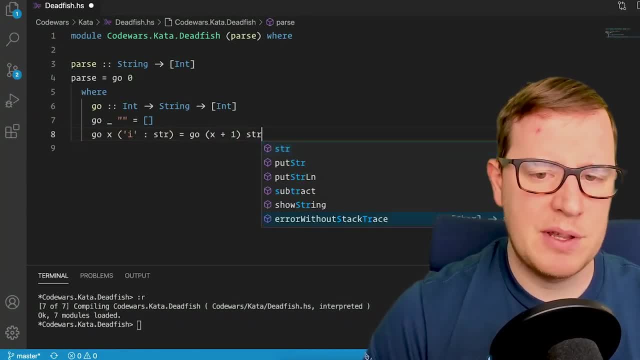 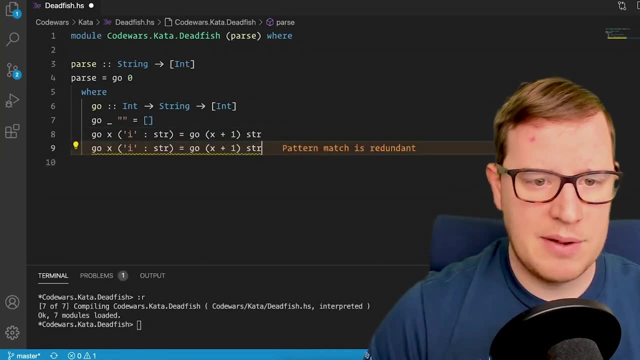 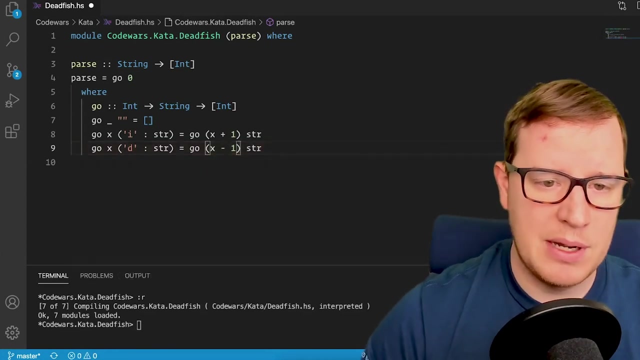 to parse the rest of the string And the rest of the commands are going to be very similar to this one. So, for example, let's handle now the decrement- When we pass the D is going to do x minus one And, if you're noticing, since we are using the conservator in Haskell, 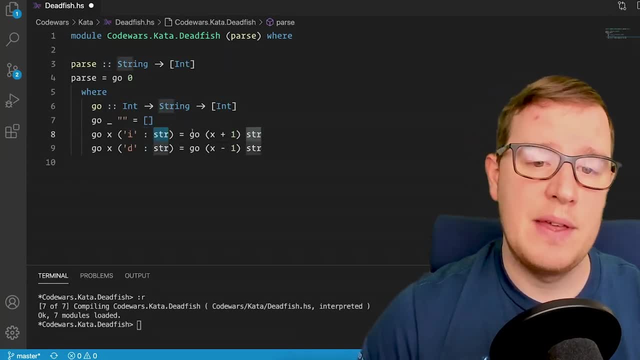 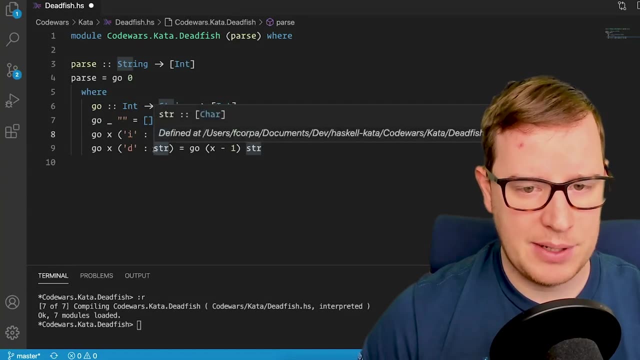 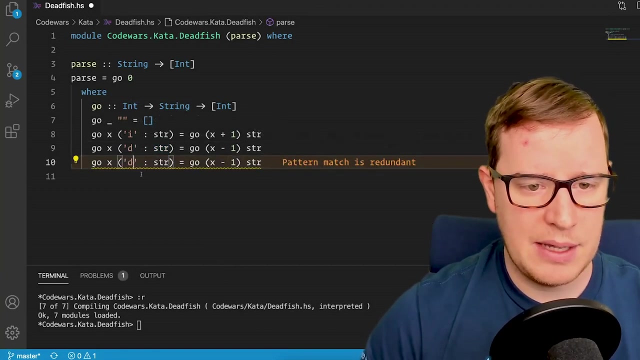 we're actually removing the first chart of the string and then recursively continue with the rest of the function, with the rest of the commands that might be might end up in the string. So now we handled our decrease case as well, And now let's handle the s case. 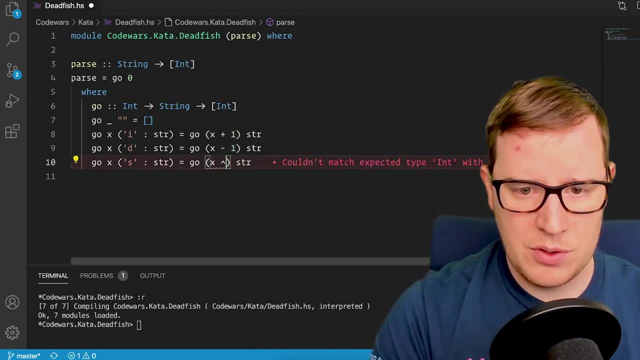 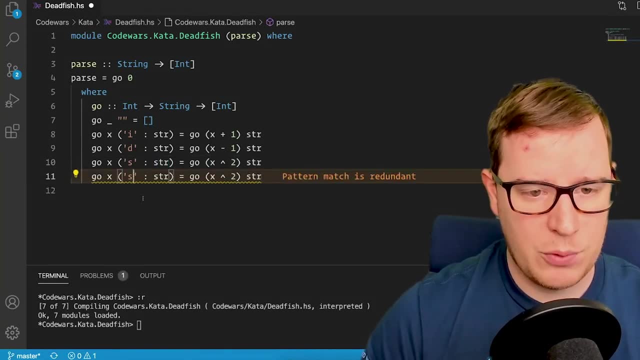 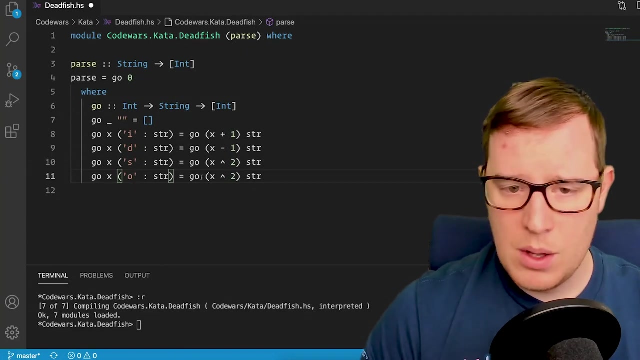 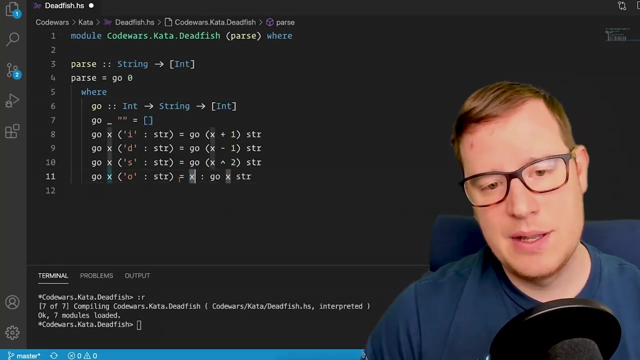 In this case, we're going to do x by two And then we want to handle the case in a way which we said it's going to append to the end. Well, in this case we can use the conservator back And obviously we are adding now to the end result the the state that we used. 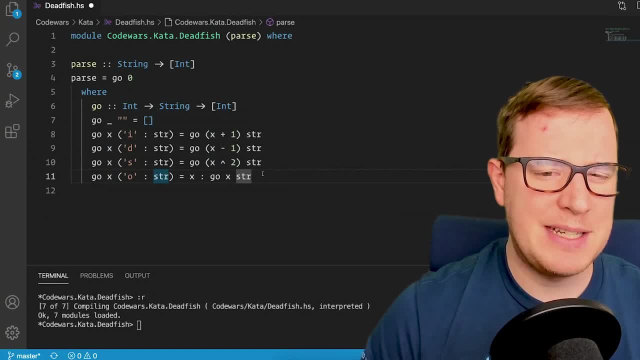 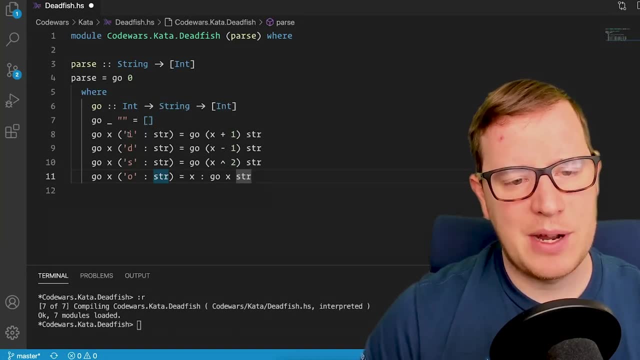 to have the next element. Okay, so it seems that we handle all of the cases, but now we're not really, because if we output this to code wars, it will complain and it will try to fail with other commands that are not any of those. So how do we handle this? Well, 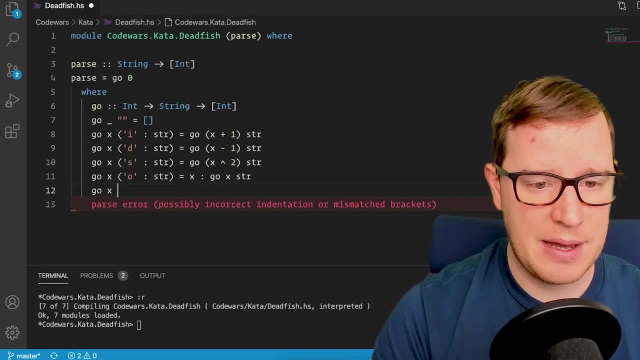 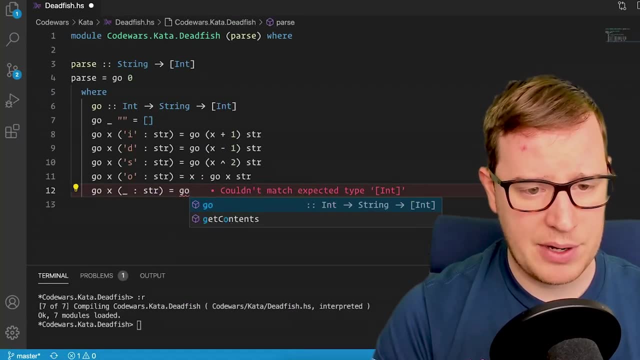 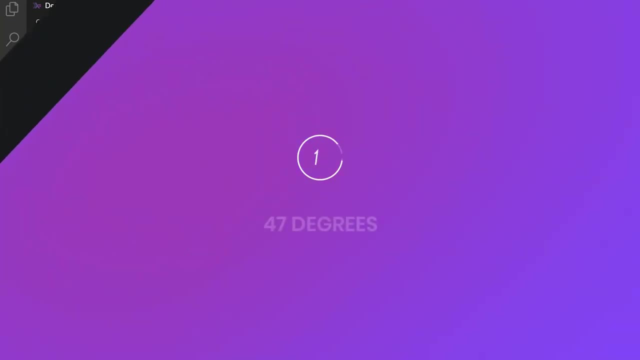 since we are a pattern matching in Haskell and pattern matching is awesome, we say that for any other command. we're just going to ignore it and keep the recursion going. Okay, so let's load this up in our REPL. Let's check it out. 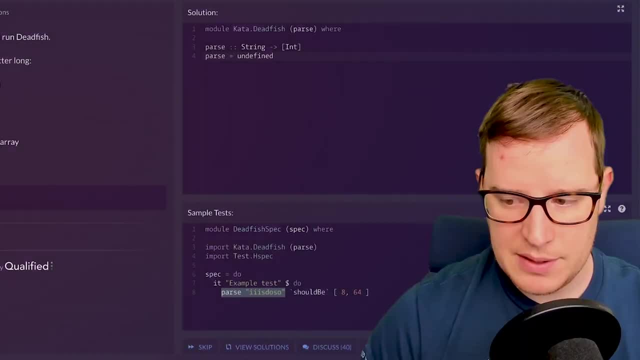 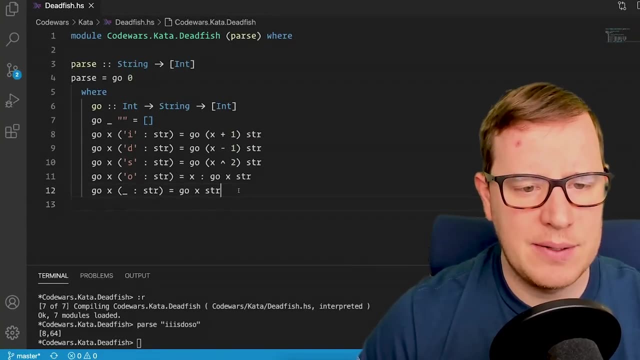 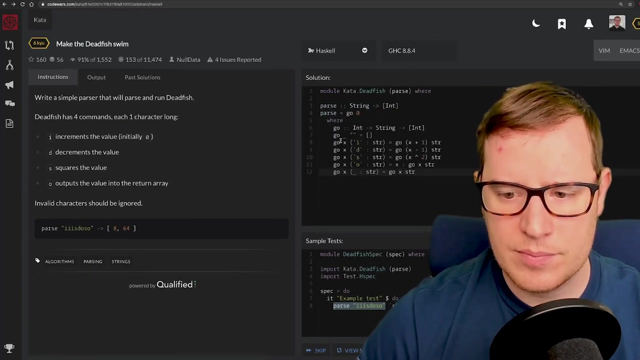 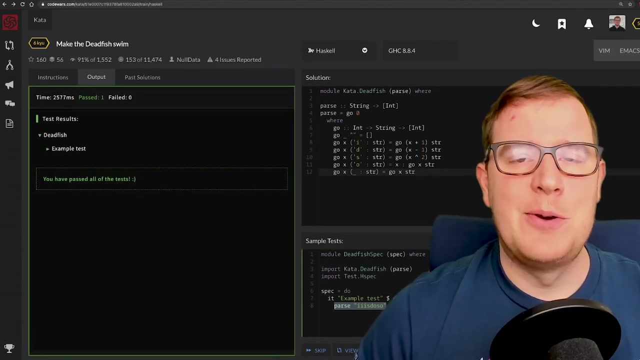 Okay, so let's load this up in our REPL. Let's check it out This. we're going to parse this and see what happens. Awesome, So it seems that it's working. Let's try it out in code wars And see if we are good to go Test. Nice, So it looks. 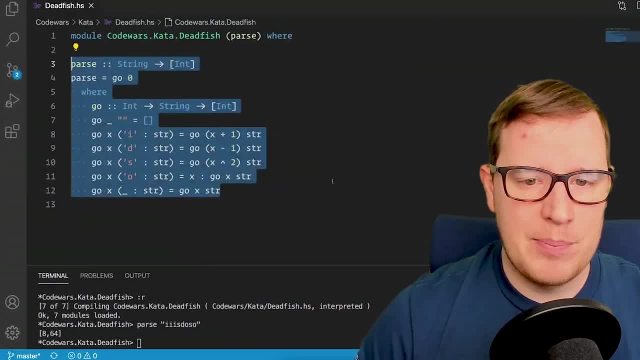 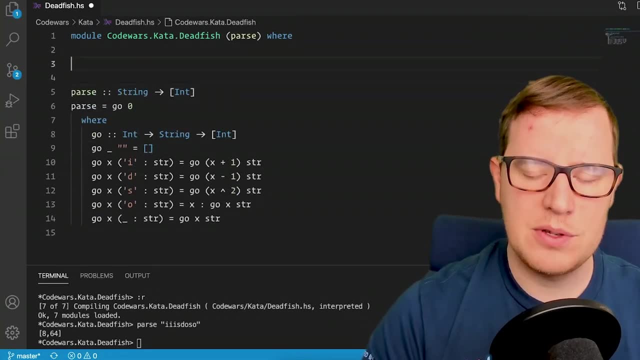 like we did it. But let now let's get a bit more fancy. We're going to do something similar to this, but not quite exactly. we're going to use a monad called rws, which is like a sum of the read monad, the reader monad, the state monad and the writer monad. So you can import it either from: 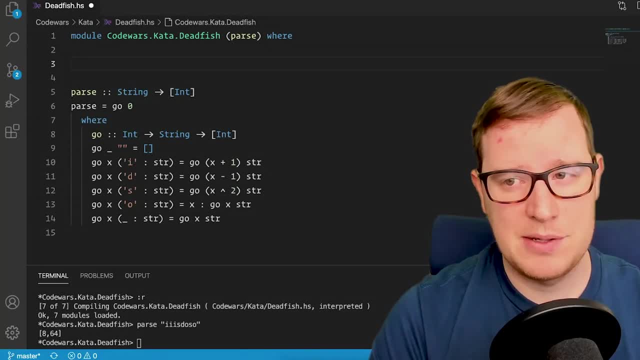 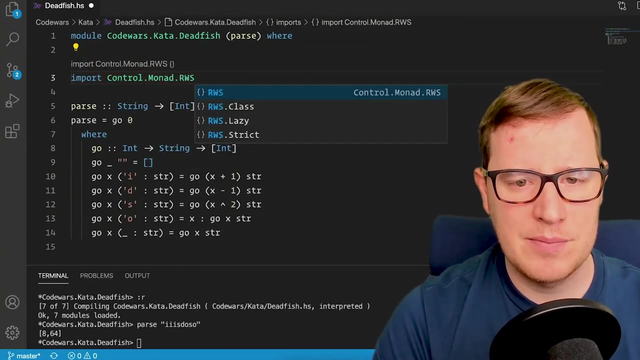 NTL or transformers. I'm going to use MTL because the input looks nicer. So import control monad rws. Let me know if I know how to spell control monad rws. And we are going to import rws monad. 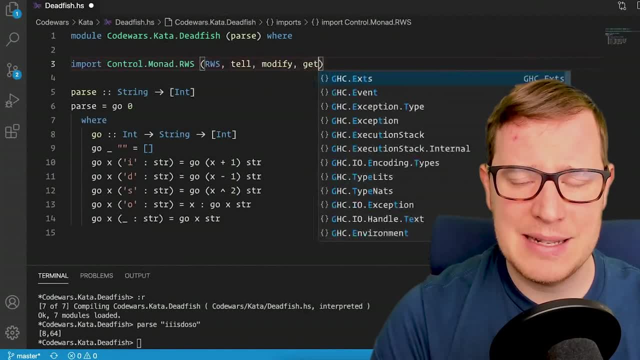 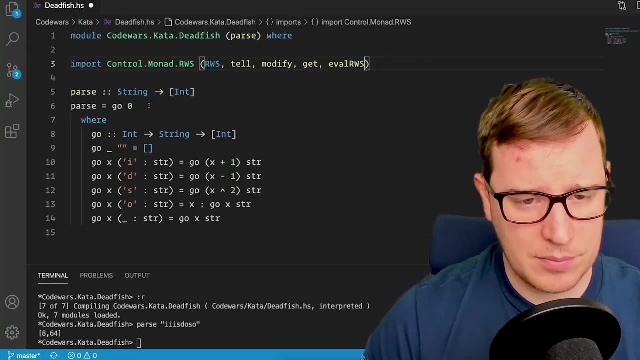 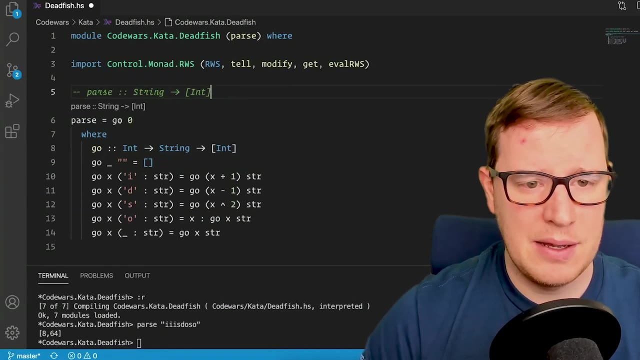 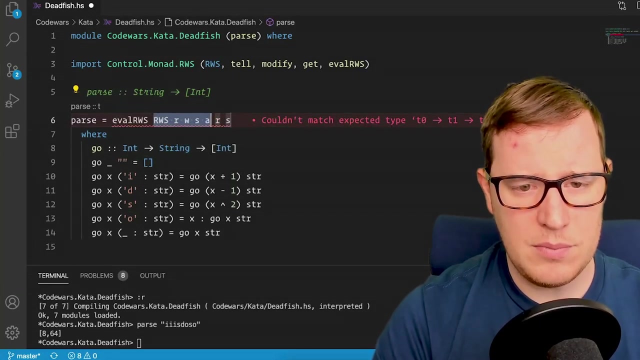 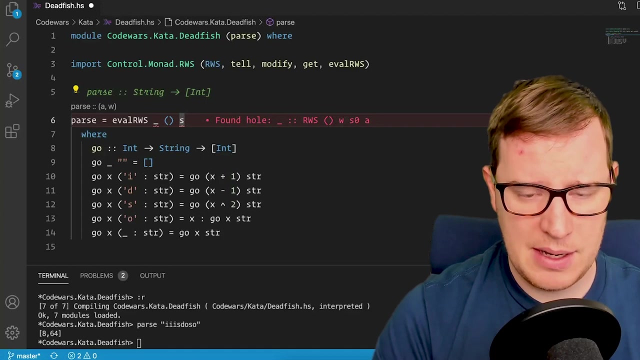 tell, modify, get and eval rws. I think this is all we need And for now, we're going to ignore this And say that we're going to eval our rws with some function. The read, the environment for the reader, monad is an empty tuple, is nothing and the state is going to be zero. So let's have a look, Let's. 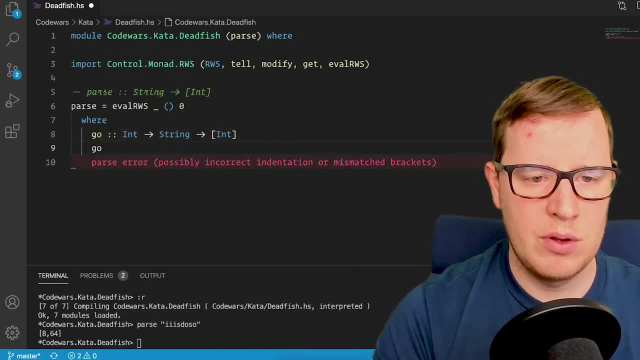 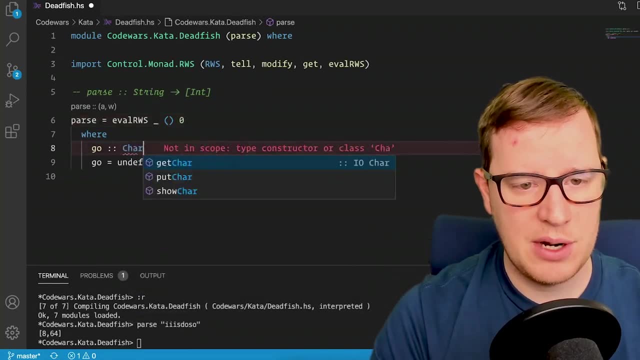 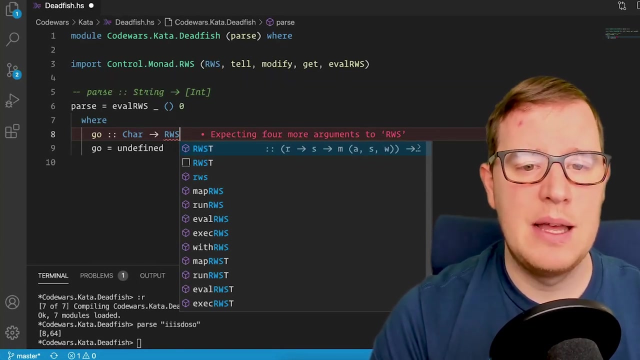 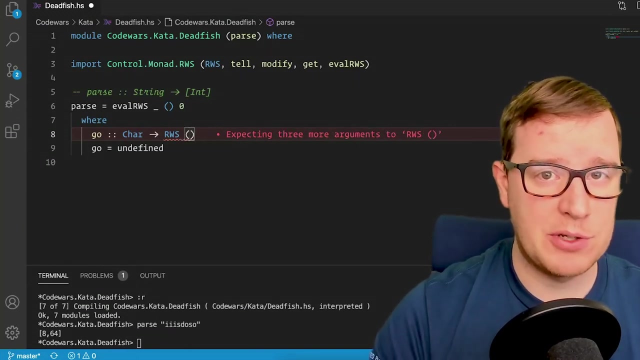 remove this for now And defined- And here we want a function that it's going to take a char and it's going to return the reader. writer, state monad And the. the reader environment that we're going to provide is nothing, because we're not going to. 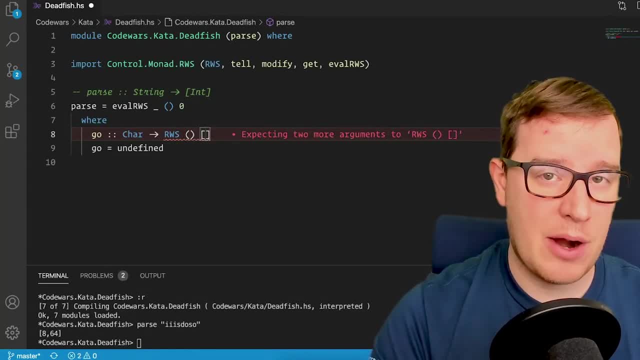 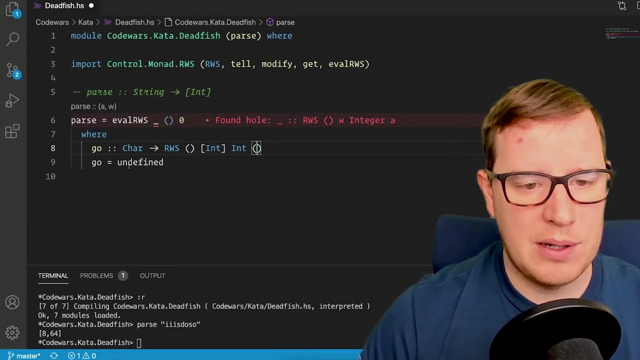 use the reader moment here. The writer state is: our end result is going to be a list of int. The state that we want to accumulate, that start by zero is going to be an end, and then we need to find an end with an empty tuple. So how does this work? Well, 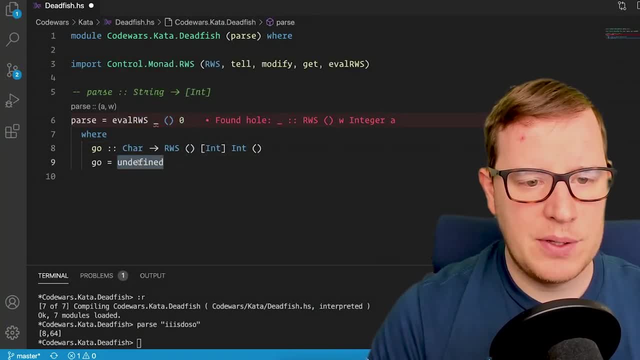 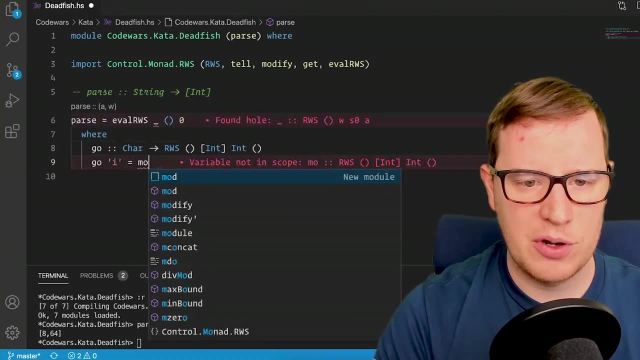 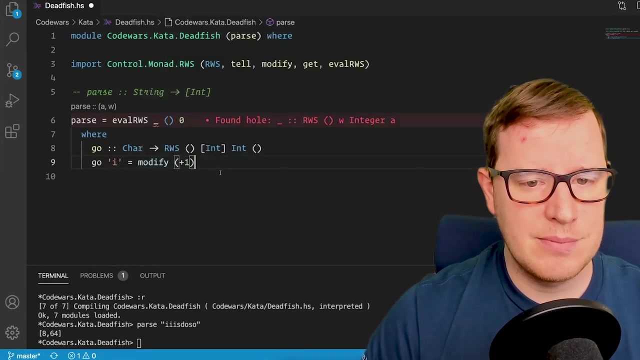 let's handle all the cases first. And we're going to say that, in case our command is I, we're going to call the function modify with plus one- Awesome. In case our command is D, we're going to apply the flipped version of minus of one, great. 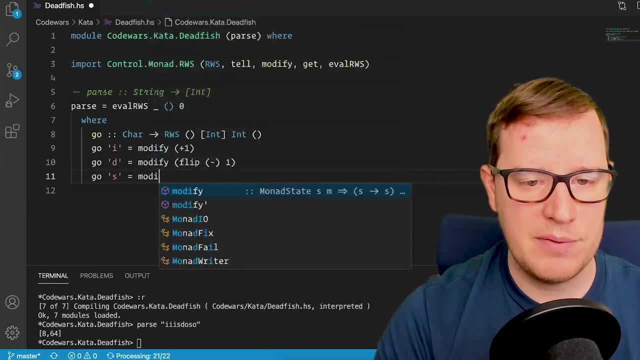 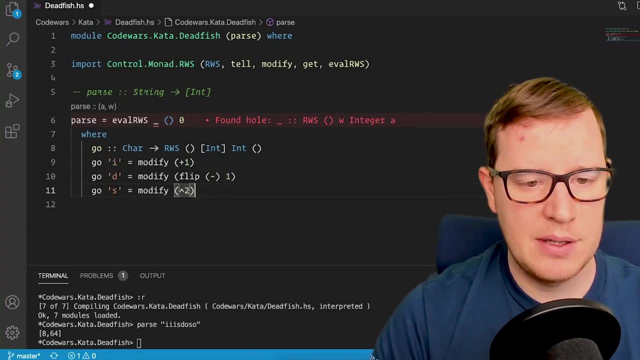 in case is an S. we want to also call Modify, calling the function Exp grateful וב icip in. in if we were to apply of minus, we create a null in caseassemble an S. Whatever this 3000 is going to be, we're going to call the function create salud mode U against the plus 1.. 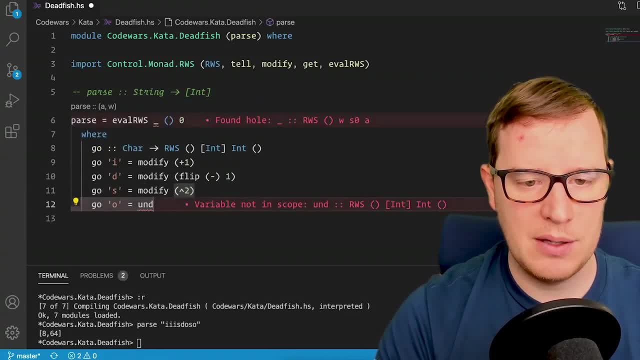 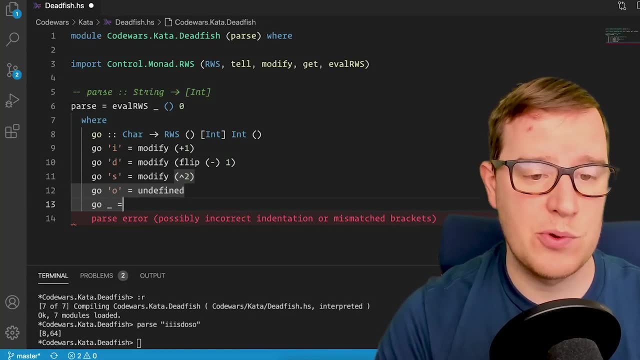 In case it's an O, we're going to do something else. And what happens if it's any other command? How do you tell the monad to don't do anything? Well, to just do pure unit. because we are in the context of a monad. 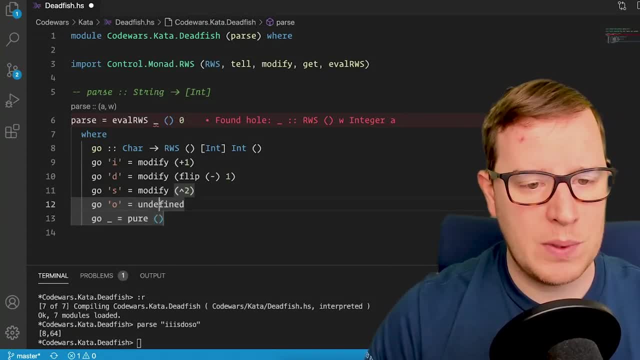 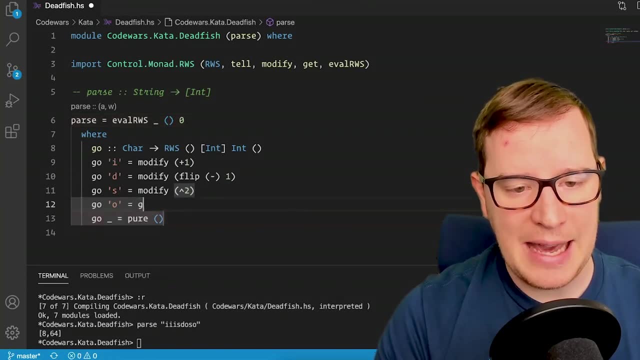 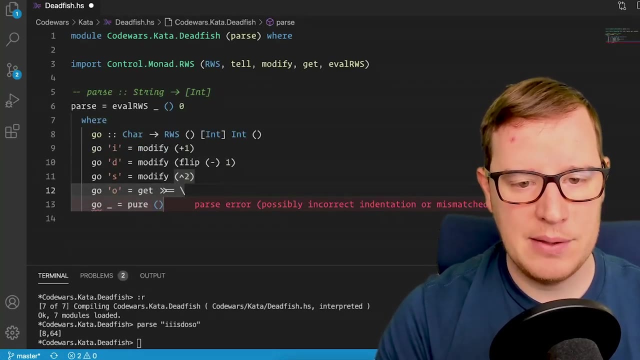 So this computation will do absolutely nothing. So what happens in the O case? Well, in the O case we need to get the value that we have from the state monad, And now we need to pipe it into a lambda that we're going to call n. 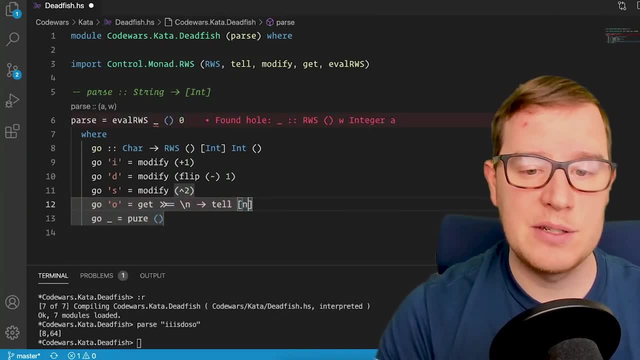 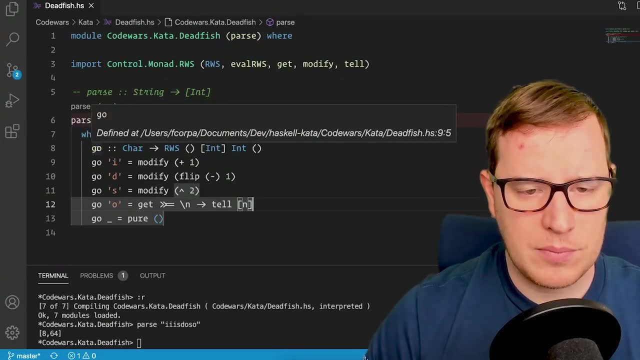 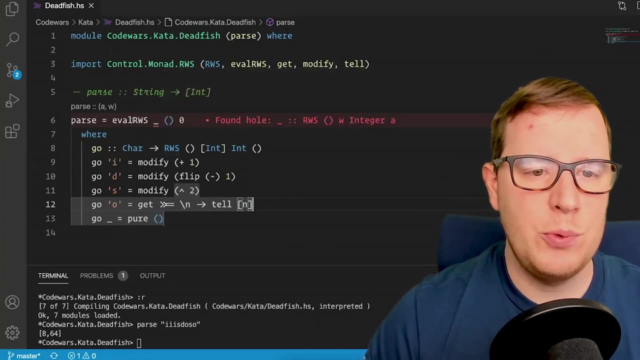 And then we're going to tell the writer, monad, to add a list with that element. Looks nice, right, Great. So now we have a function that expects a char and returns the reader. writer state: monad. But how do we use this? 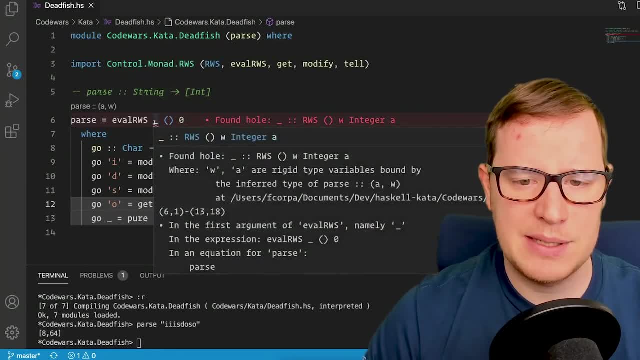 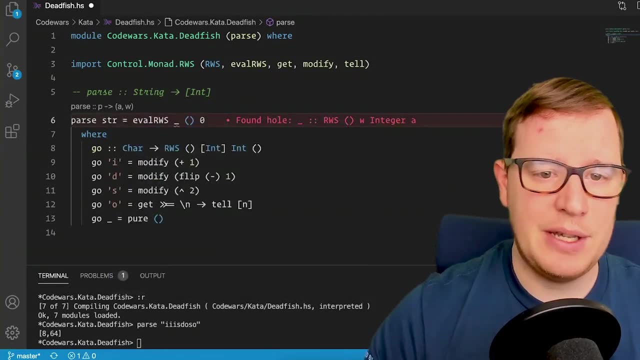 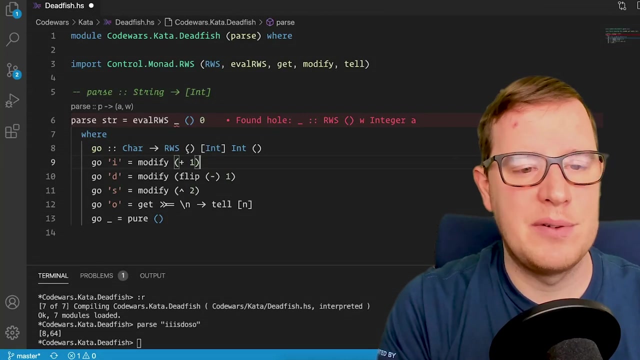 How do we run it with eval? What is this waiting for? Well, actually, if you remember, we're going to receive a string here, And then we need to apply to every character of the element this computation. So we need to accumulate a series of effects by a certain function. 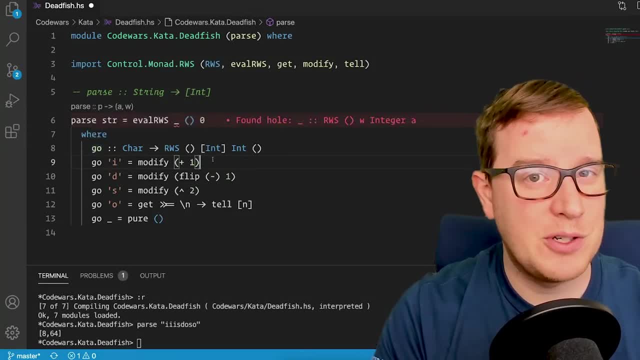 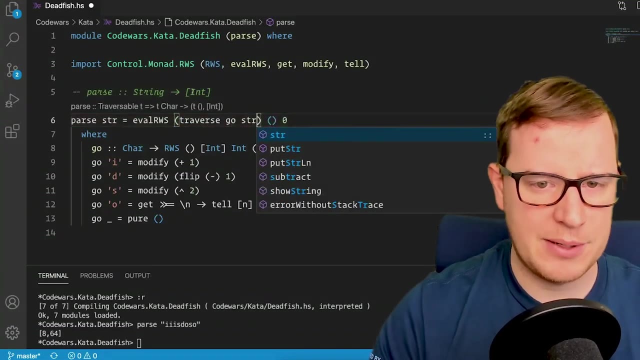 This is the function that we're going to use, But what function do we always use when we want to apply a series of effects and accumulate them somewhere? Well, you guessed it right, It's our dear friend. traverse By the function. go with all the string. 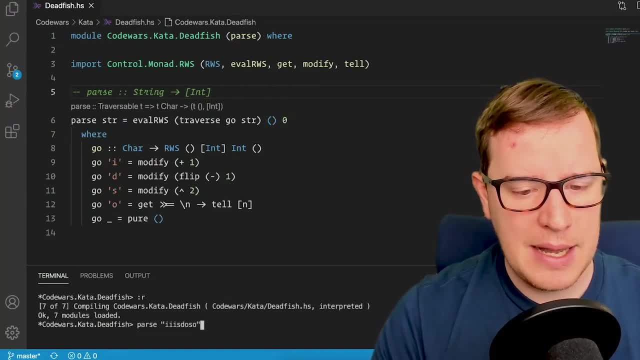 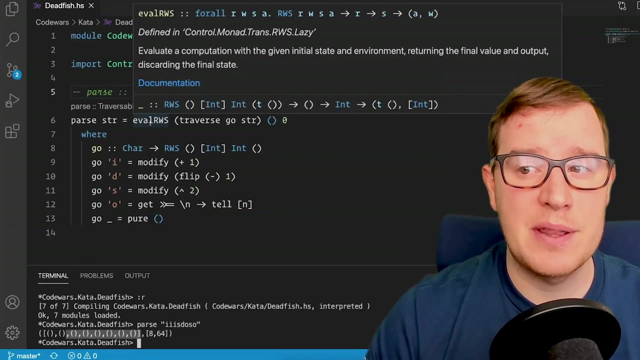 Great. So let's see if this is compiling Looks good. And now what happens if we call parse? Oh, interesting, So we're accumulating everything. So you see, eval returns evaluate a computation with a given initial state and environment, returning the final value and output, discarding the final state. 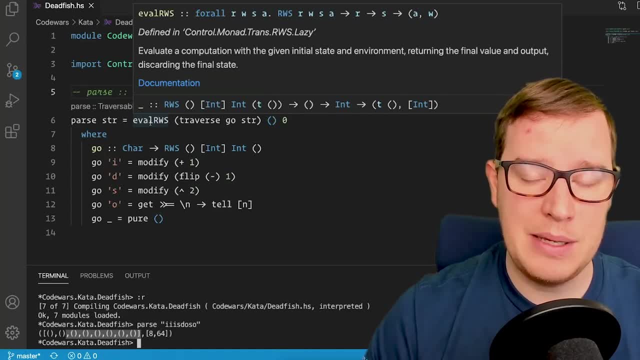 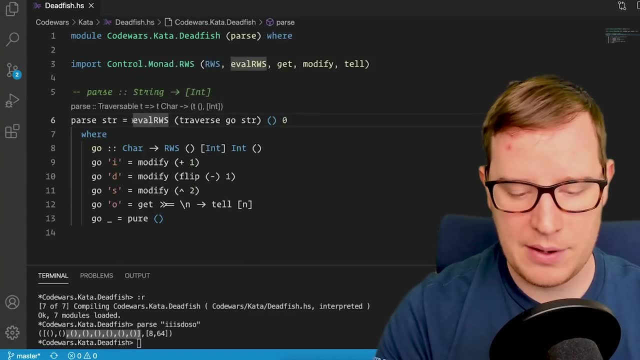 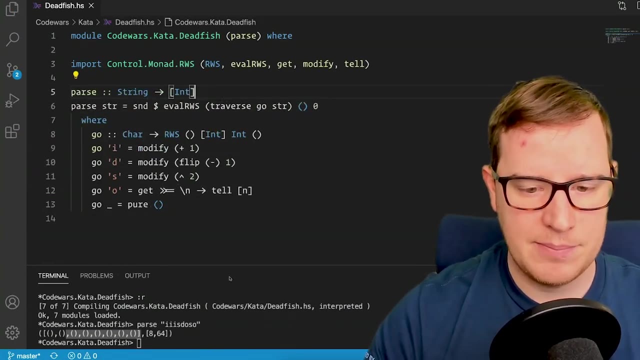 So what we really want is the output, but we're being returned a tuple with the final value, which we don't care about, and the output, So we need to append here. second, from the tuple functions. And now our type signature is correct again. 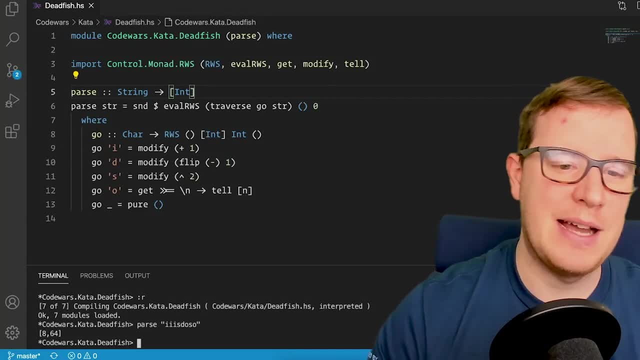 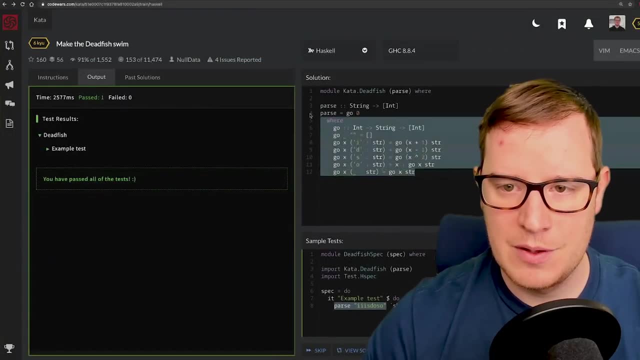 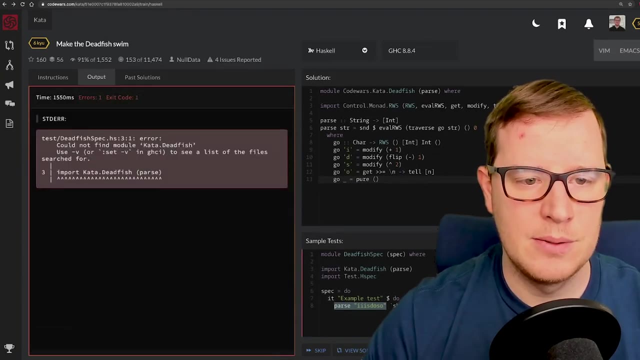 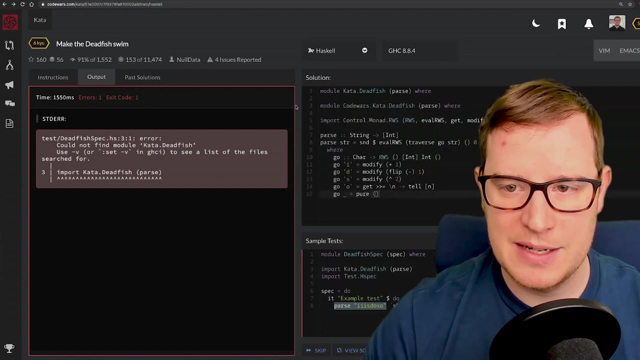 Let's see: Great, And this worked. exactly the same. Let's check it out in code wars and see if it works. Test Oops. Okay, I messed up this, So the name is not exactly the same as my environment. That's to be expected. 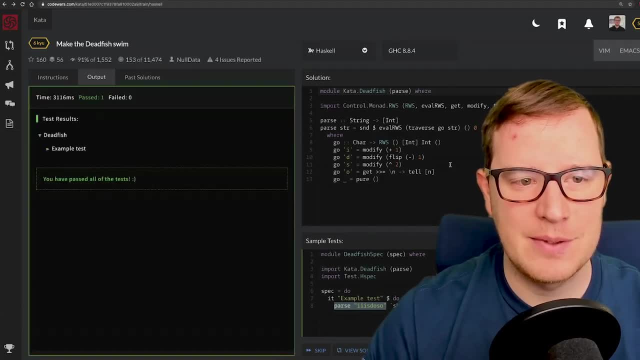 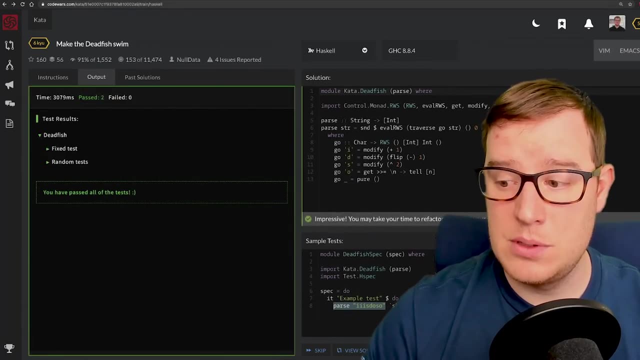 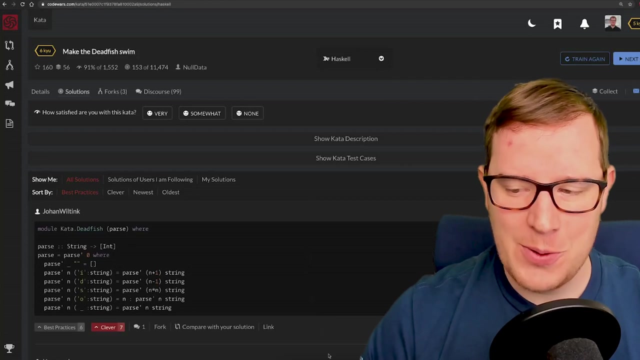 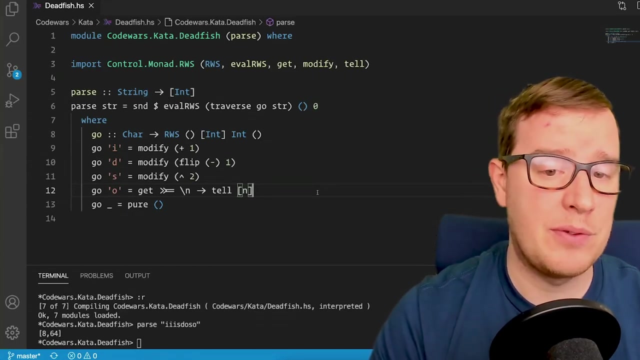 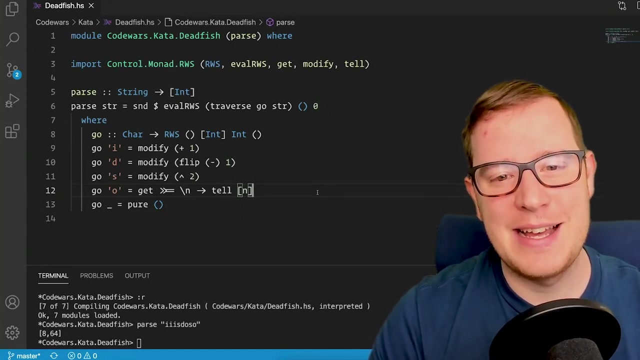 The module is different. Let's try it now. Awesome, And now for the final run. Not final yet Great, So it passed. So, as you see, we can pretty much resolve any looping problem in Haskell with recursion, But sometimes it's nice if we use of this. Kirky monads like reader and state and writer. 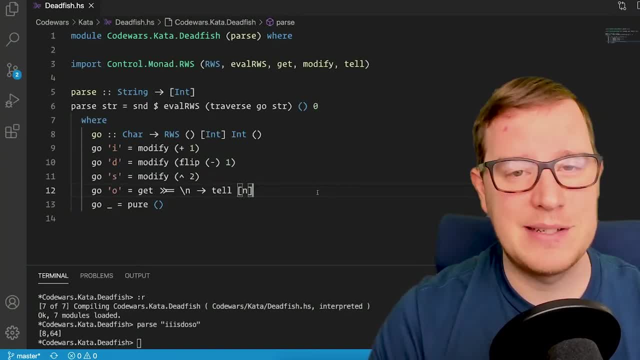 And if we combine them all in the RWM we get the same result. So if we use the RWS monad, the solution is quite nice. Obviously this is an overkill for this problem, but I thought it might be a nice exercise on the features. 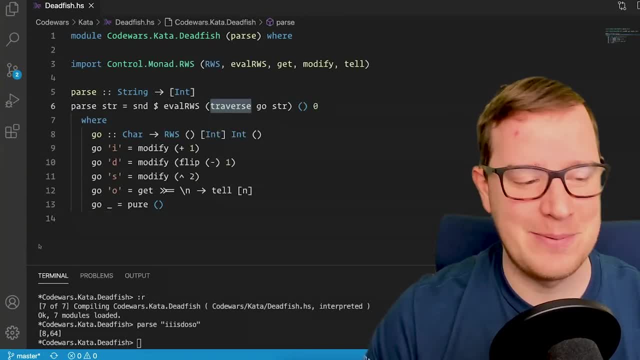 Our favorite function traverse. So I hope you enjoyed the video and see you next time.